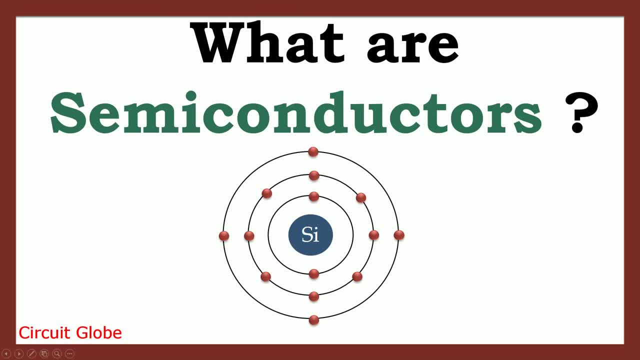 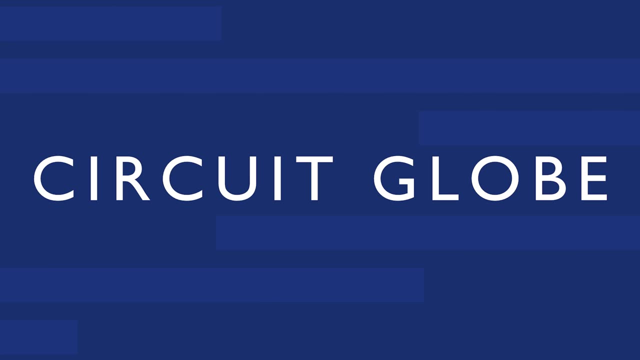 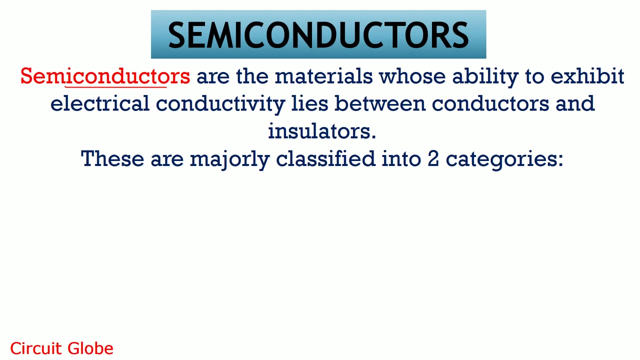 Hello everyone, once again, welcome to Circuit Globe. I am Roshni and in this session we will be going to discuss what are semiconductors. So, friends, let's get started. So friends, basically, semiconductors are those materials whose ability to conduct lies between: 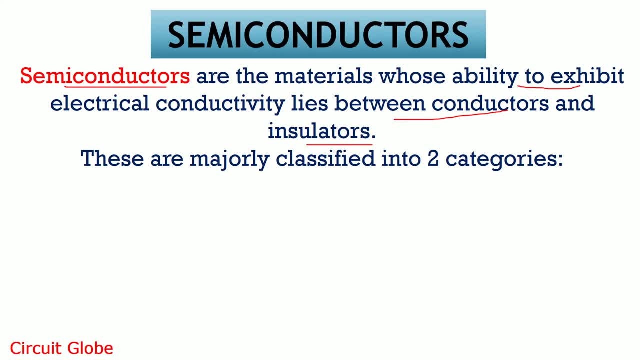 conductors and insulator. We are already aware of the fact that conductors are basically those materials which possess good electrical conductivity, As against insulators are those materials whose electrical conductivity is good. So, friends, let's get started. So, semiconductors are basically those materials whose conductivity is somewhat less than conductors. 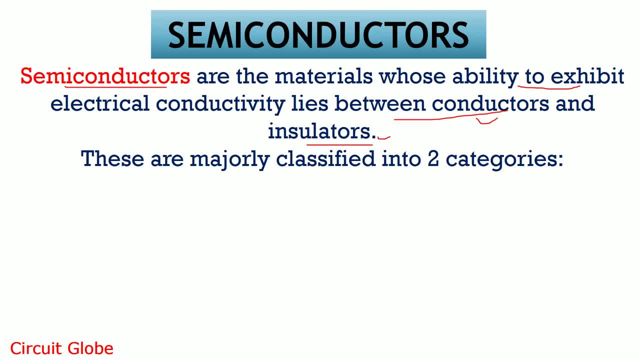 but it is very much higher than an insulator. So semiconductors are majorly classified into two categories. First one is intrinsic and the second one is extrinsic. Further this extrinsic semiconductor is classified into N type and P type, And we will discuss these. 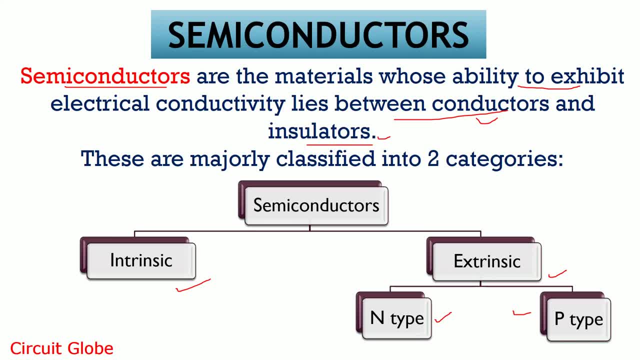 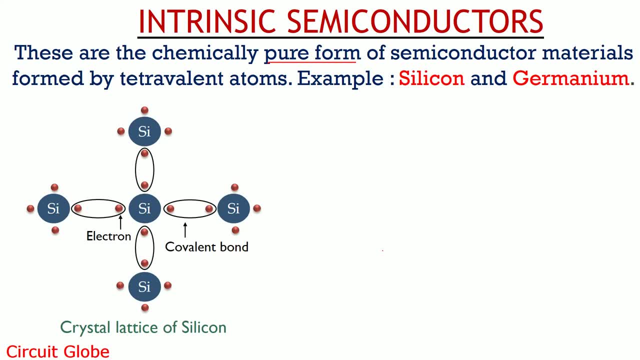 two type in detail. Let's first understand what are intrinsic semiconductors. Intrinsic semiconductors are pure form of semiconductor materials and these are formed by tetravalent atoms. And we know tetravalent atoms, or group 4 elements, contains 4 electron in its valence shell. The examples: 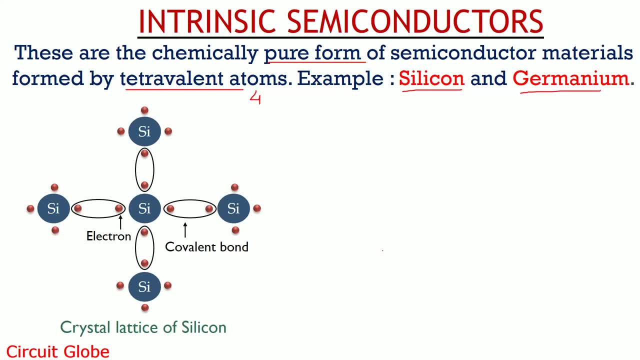 are silicon and germanium Here. the figure clearly shows the crystal lattice structure of silicon and germanium. Here each silicon atom forms covalent bonds with the other silicon atom present in its neighbouring area, And it do so by making use of electrons present. 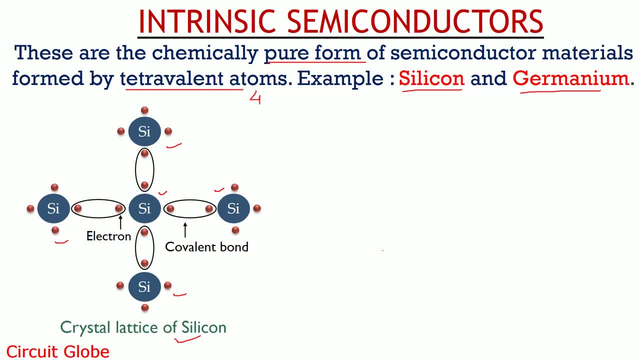 in valence shell. These electron in the valence shell of silicon atom forms covalent bond with its neighbouring silicon atom, And at room temperature these electrons are bounded closely with each other, But once some external heat is provided, these electrons are bound together, So in the form of electron electron is created and in a vacuum Electrons gain. 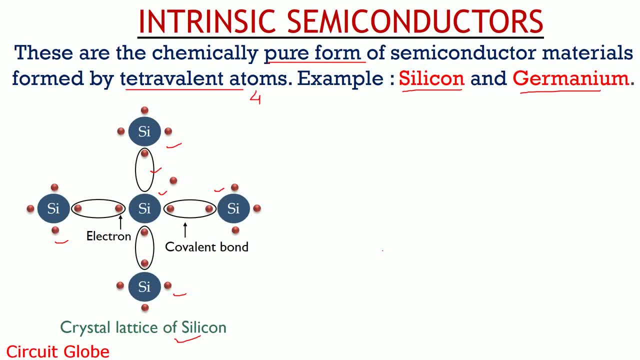 sufficient energy and leaves its position. At that particular point of time, a vacancy of electron is created, which is termed as hole. However, this movement of electron generates conduction through semiconductors. Let's now have a look at the energy band diagram of intrinsic semiconductor, As we have recently. 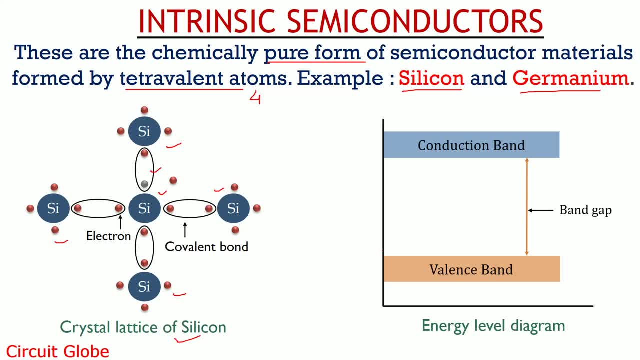 discussed that with increase in temperature electron leaves its position vacant and gets free. Here also we will discuss the same criteria with the help of energy level diagram. So basically, the electrons are present in valence band, but once some external heat is provided, so with the increase in temperature, these electrons get free and moves to conduction. 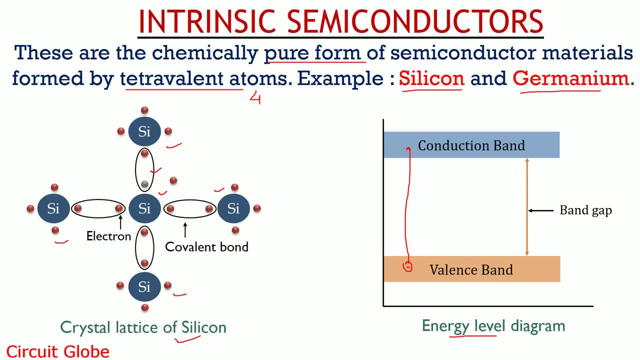 band, thereby causing conductivity to increase and resultantly, this causes resistance of semiconductor to decrease. basically, this band gap is nothing but that particular energy which is required to get the electron free. with further increase in temperature, more electron from valence band moves to conduction band, thereby increasing the conduction of. 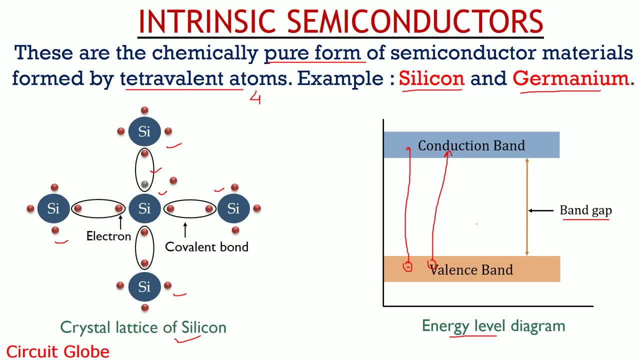 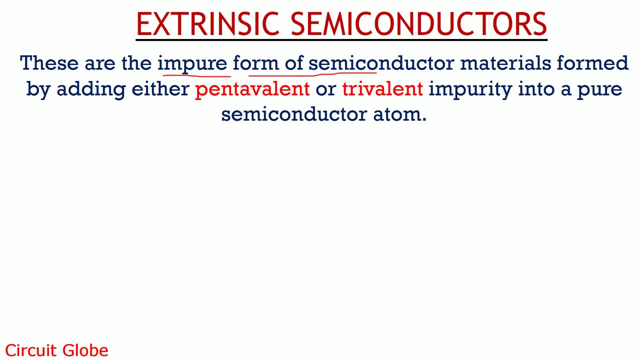 the device. Now, friends, after having idea about how intrinsic semiconductor conducts, lets move further to understand the same for extrinsic semiconductor. Extrinsic semiconductors are basically impure form of semiconductor materials, and these are formed when we add either pentavalent or trivalent impurity to a semiconductor material. 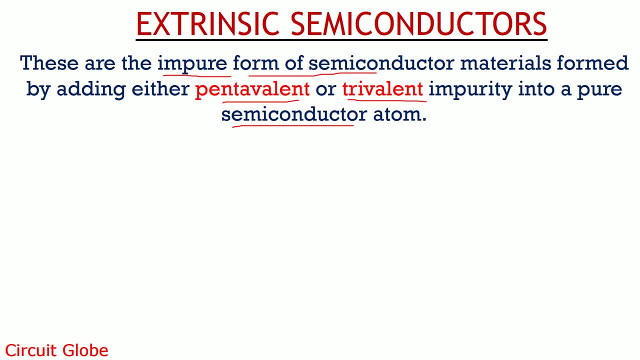 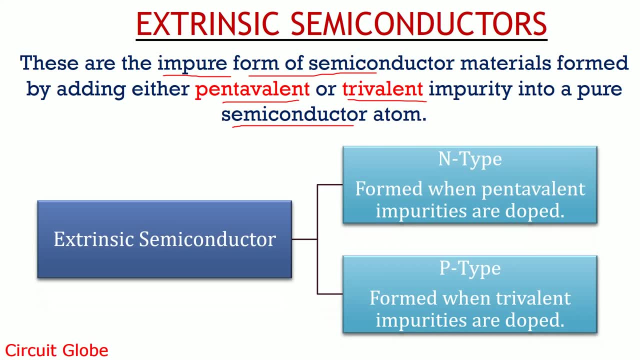 which is in pure form, or we can say a tetravalent silicon or germanium atom. Now just have a look. what are the types of extrinsic semiconductors? So extrinsic semiconductors are basically of two type. The first one is n type and the second one is p type. 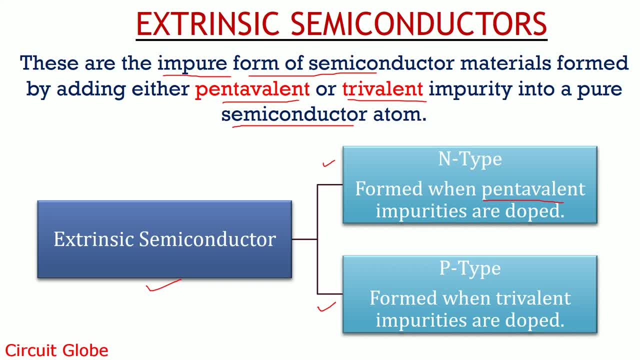 n type extrinsic semiconductors are formed when pentavalent impurity or group 5 elements are doped to a pure semiconductor atom. And p type semiconductors are formed when trivalent impurity or group 3 elements are added to a pure semiconductor atom. 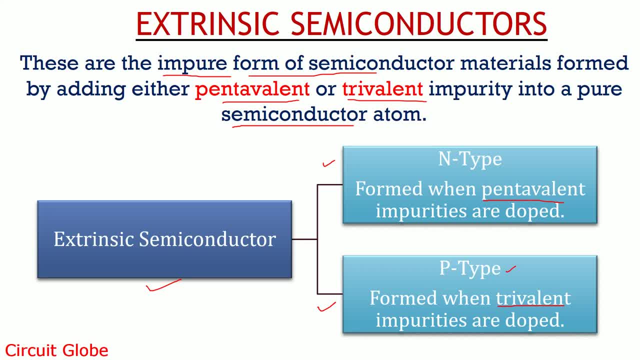 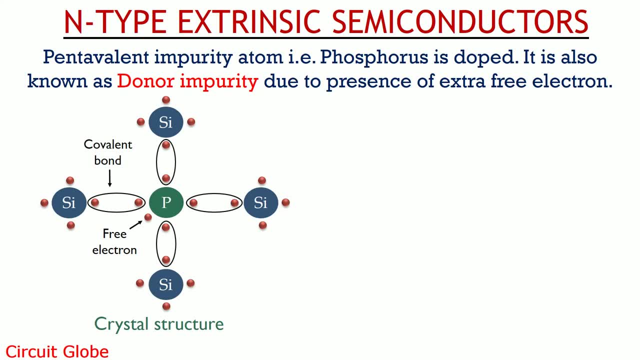 So lets first discuss what is n type extrinsic semiconductor in detail, As we have recently discussed That n type extrinsic semiconductors are formed when pentavalent impurity or group 5 elements are doped into a pure semiconductor material. 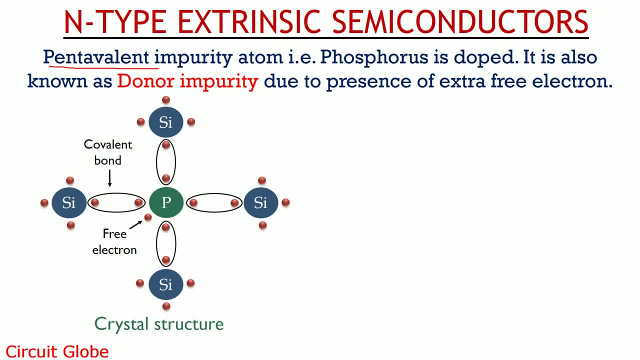 For example antimony, bismuth or phosphorus, And here we have used phosphorus atom to be added into a pure silicon structure. We know that group 5 elements contain 5 electrons in its valence shell. So the 4 electrons of phosphorus form 4 covalent electrons. 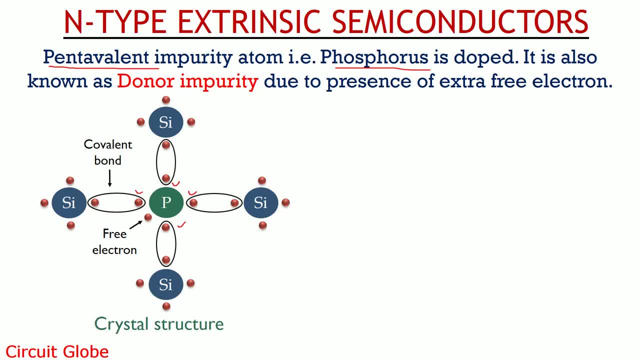 So the 4 electrons of phosphorus form 4 covalent electrons, And 3 electrons of phosphorus are covalent bonds with its neighboring silicon atom, But still a free electron is left which is unbounded and is responsible for conduction. 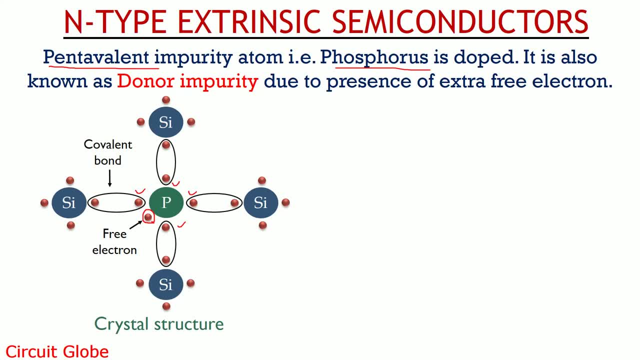 further, when some external heat is provided, like in case of intrinsic semiconductor, electron breaks the covalent bond and leaves its position vacant, thereby creating a hole. This somewhat increases the conducting level of semiconductor from covalent bonding to semiconductor, more in case of extrinsic semiconductor than in intrinsic semiconductor. These are: 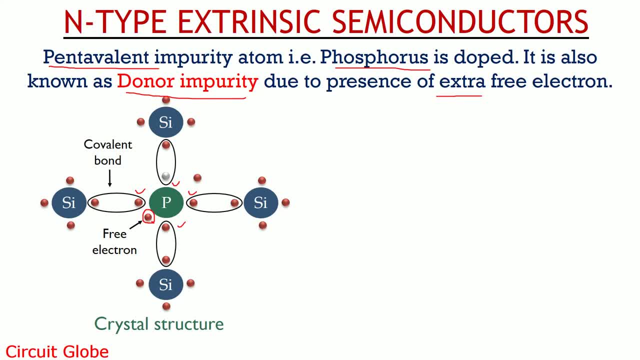 also known as donor impurity due to the presence of extra electron. Let's now have a look at the energy band diagram of n-type extrinsic semiconductors. Here the donor energy level in the energy level diagram shows the energy level of free electron present in the crystal. 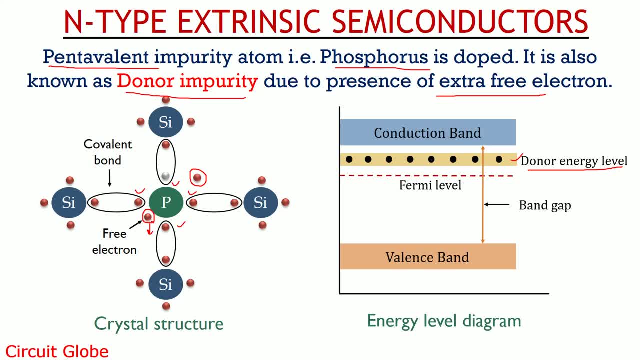 These electrons have sufficient energy, even at room temperature, in order to reach the conduction band and thereby decreasing the resistance and increasing the conductivity. Ok, now the question arises why n-type extrinsic semiconductors are called so. The reason behind this is that n-type semiconductor contains extra negatively charged particle. This is 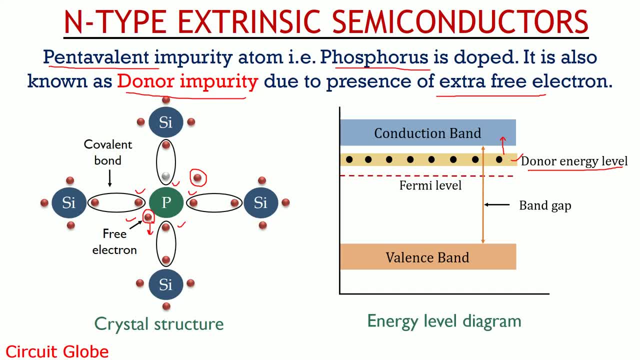 the reason why electrons acts as majority charge carriers in n-type semiconductors. Now the question arises why n-type extrinsic semiconductors are called so The reason: semiconductors and holes serves as minority carriers. Let's now have a look how p-type 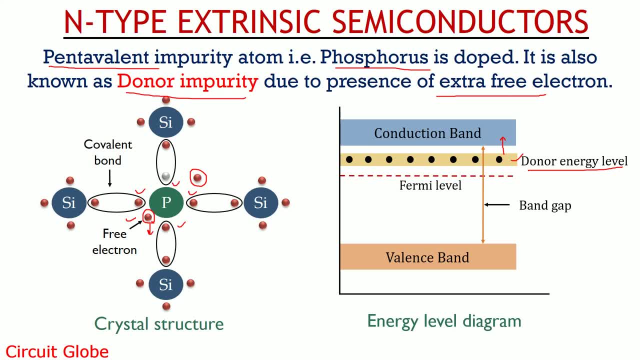 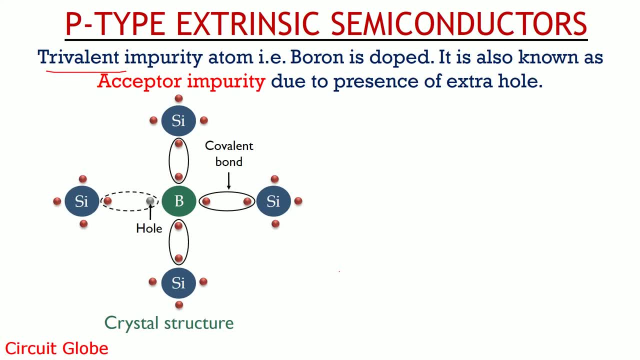 extrinsic semiconductors are formed and how they conduct. We have already discussed that p-type extrinsic semiconductors are formed when trivalent impurity atom like aluminium, indium, gallium or boron is added to a pure silicon crystal. Here we have added boron, As we know that group 3 elements.